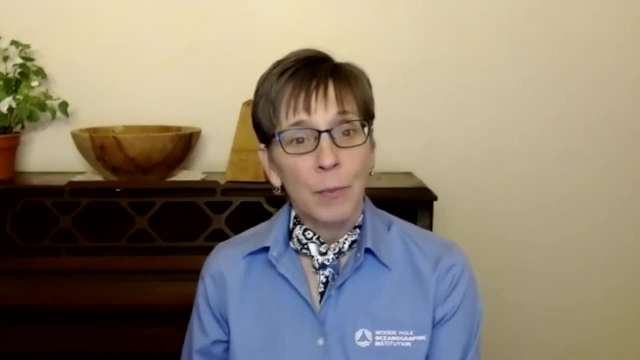 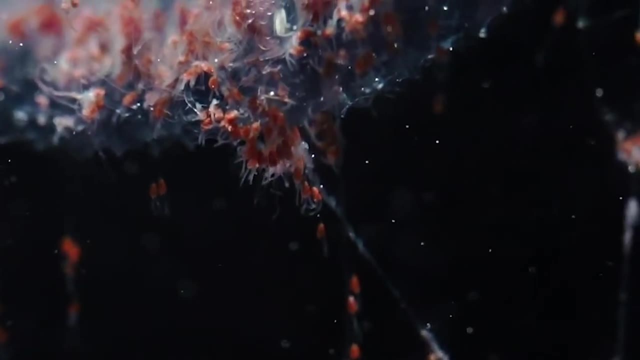 great frontiers. The Twilight Zone is a part of the ocean at the very limit of the sun's reach into the depths. It's actually defined by light, or really a lack of it. It sits below the sunlit surface, where there isn't enough light to reach it. It's a part of the ocean, that's. 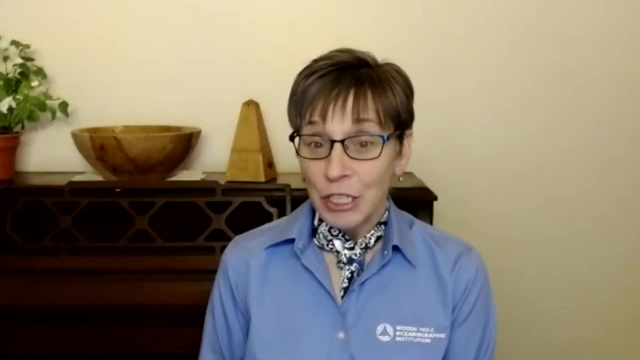 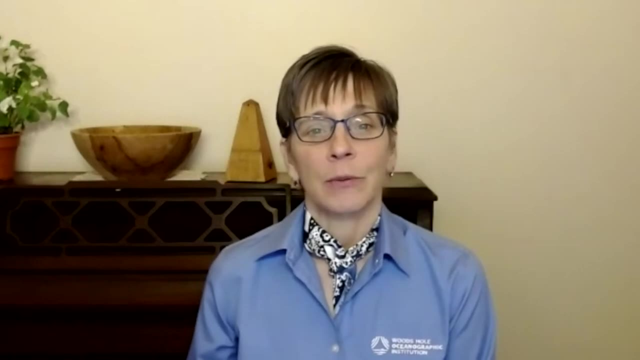 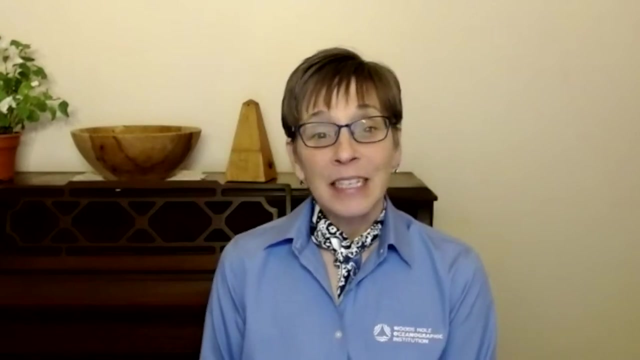 light to support photosynthesis. The depth can actually change depending on how clear the water is or even the time of day, Down deep in the Twilight Zone. conditions are incredibly harsh. It's dark, It's cold, The pressure is immense, But it teems with life. Tiny plankton, fearsome. 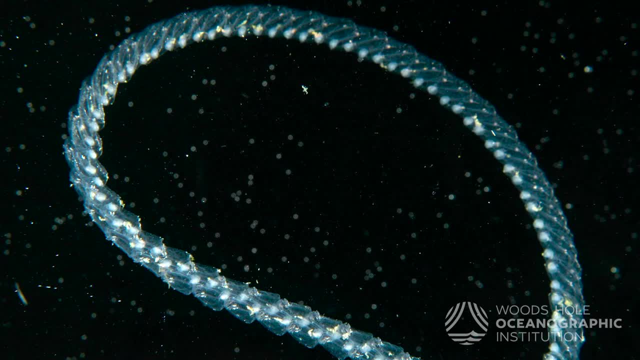 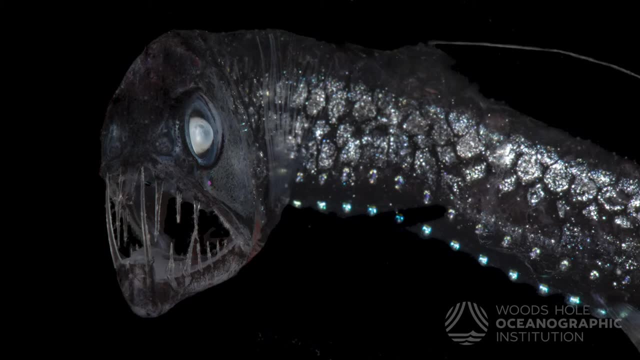 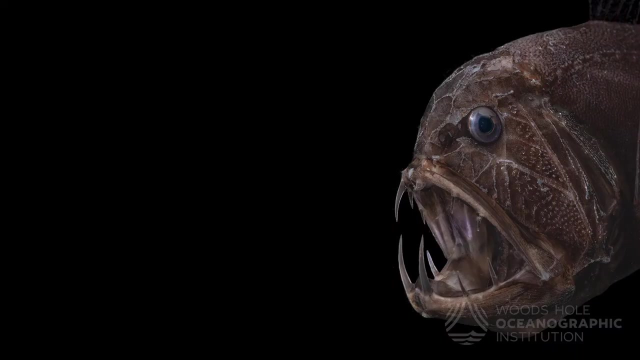 looking fish, salt chains tens of meters long. They all look a bit like aliens, but they're actually very exquisitely evolved To survive and to thrive in their home environment, just as we are in ours. You may be imagining huge. 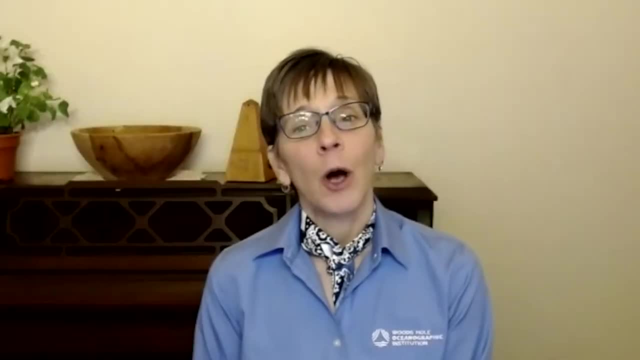 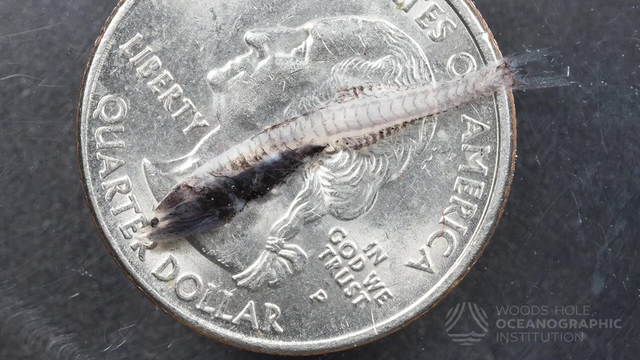 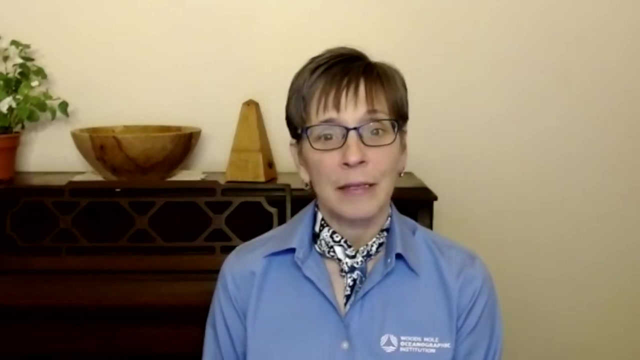 monsters lurking in the deep sea, but in fact most of the fish are about the length of my little finger. Their small size does not stop them from being powerful through sheer number. What we've learned only recently suggests that there may be as much as two or three times the fish in the 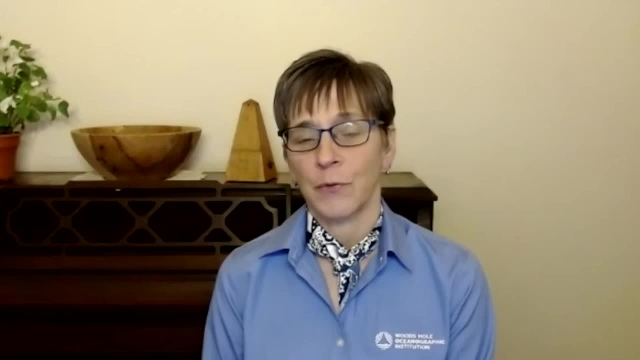 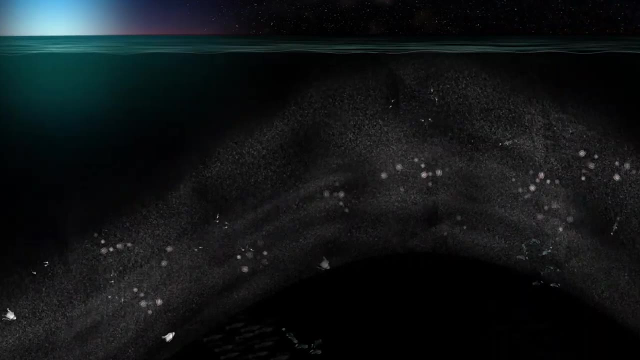 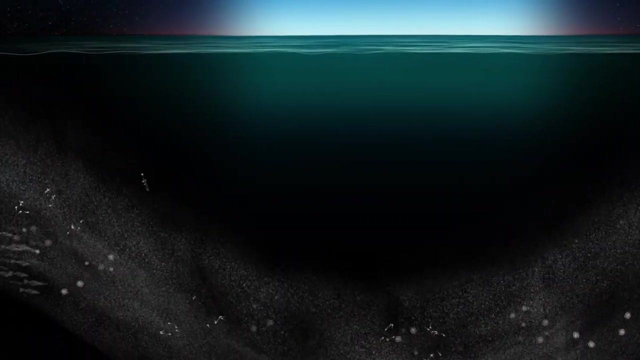 Twilight Zone. as there are in all the ocean's surface fisheries combined, The animals that live down deep migrate up to the surface to feed at night and then return to the safety of darkness during the day. That migration is the largest migration on Earth and it happens everywhere in 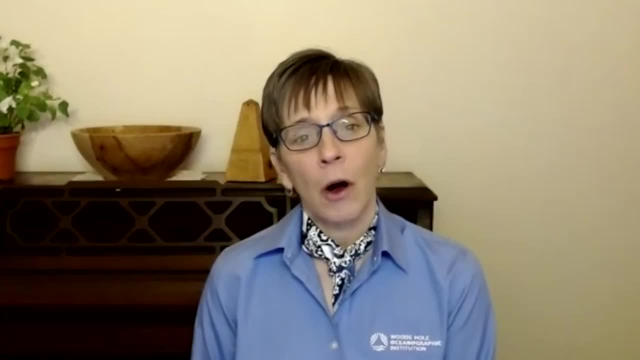 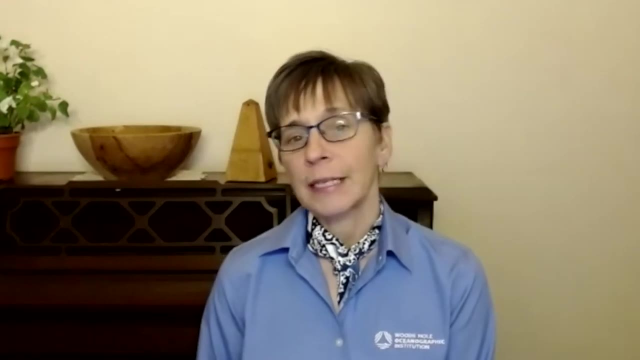 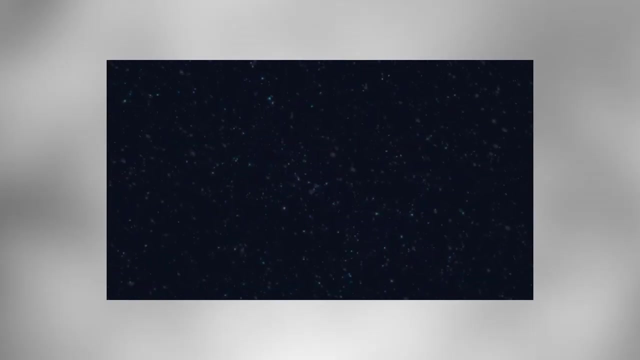 the ocean every day. That migration also helps move heat-trapping carbon dioxide from the surface water to the deep ocean. In the deep ocean it can stay locked away for a long, long time. Biological processes in the Twilight Zone are responsible for locking away two to six billion metric tons of carbon in the deep. 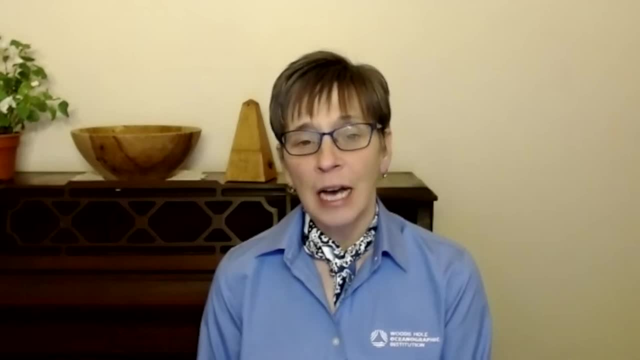 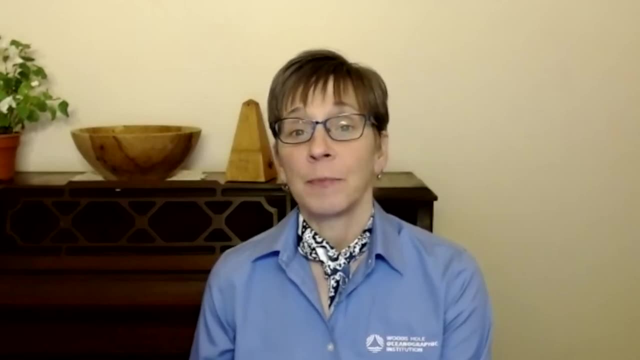 ocean each year, two to six times the amount of carbon emitted by all automobiles worldwide. All that life in the Twilight Zone is beginning to attract the attention of commercial fishers. They're not fishing in the Twilight Zone, they're fishing in the deep ocean. They're not fishing in the.